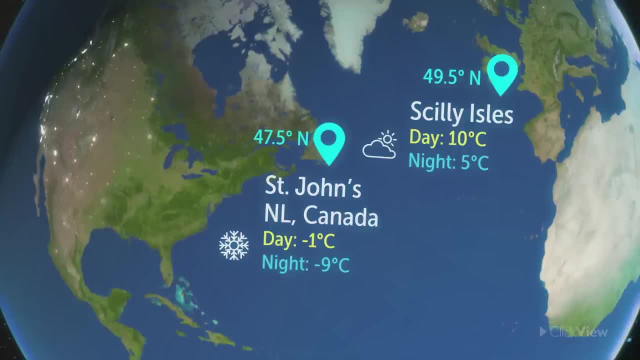 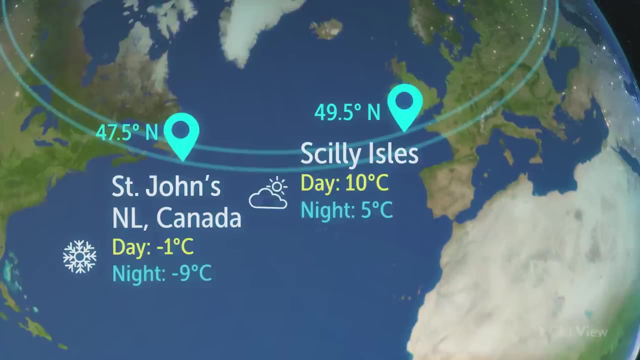 minimum temperatures at night average minus 9 degrees. That's a 14 degree difference between those two locations, even though they are at a similar latitude. One important factor is the Gulf Stream, a warm and humid area. The Gulf Stream is a very warm and humid area. It's a 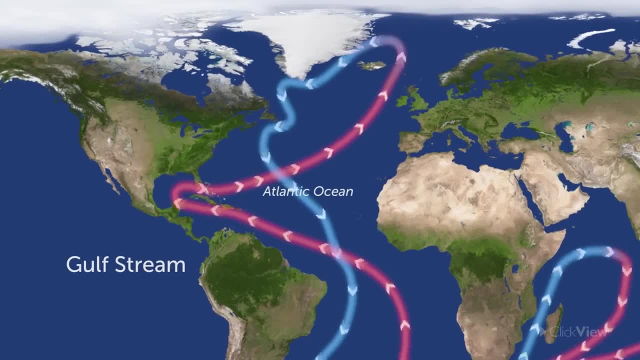 warm stream of surface water that circulates around the Atlantic Ocean. The North Atlantic Drift is an offshoot that circulates warm water around the Scillies, so the sea surface temperature almost never falls below 11 degrees in winter In St John's. at the same time, the sea temperature is: 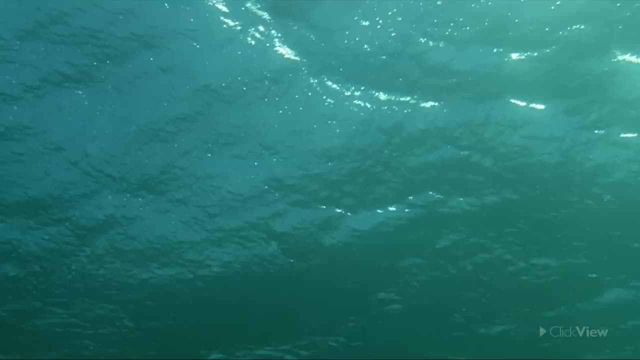 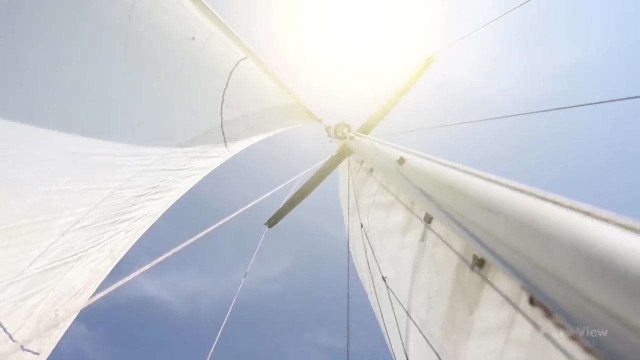 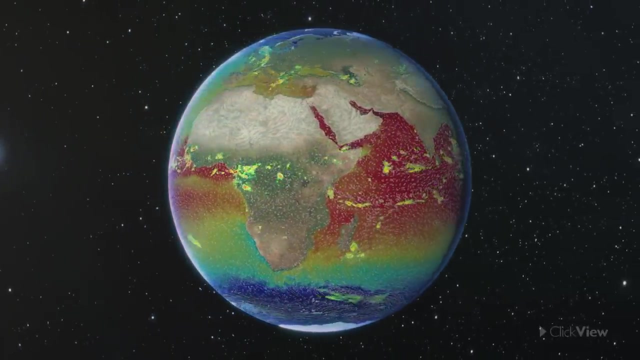 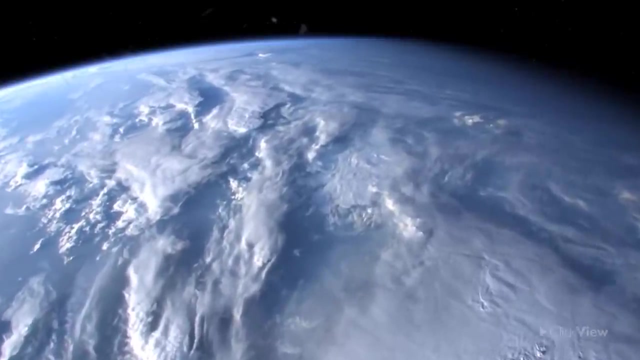 0.5 degrees. The Gulf Stream is partly caused by the circulation of ocean waters, but is mainly driven by winds. The Earth's climate, ocean currents and global atmospheric circulation or large-scale winds are interconnected. At any one time, there are many different weather systems, creating localized conditions around the globe. 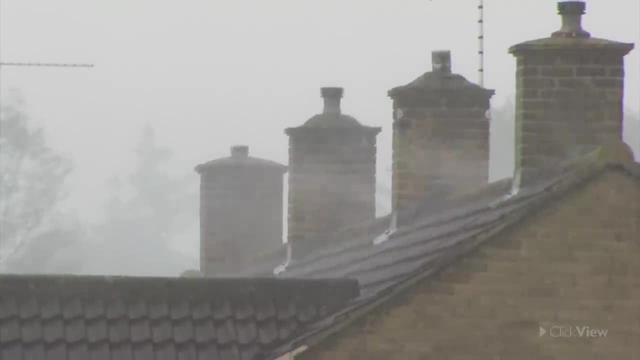 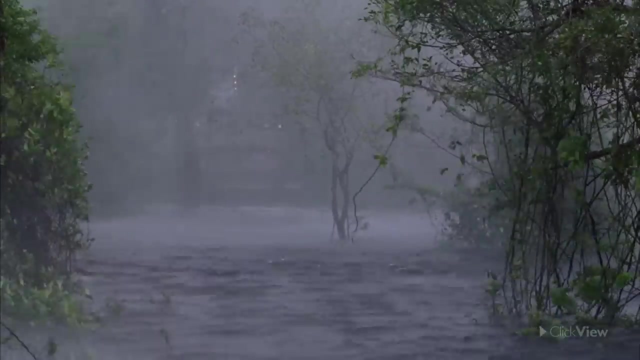 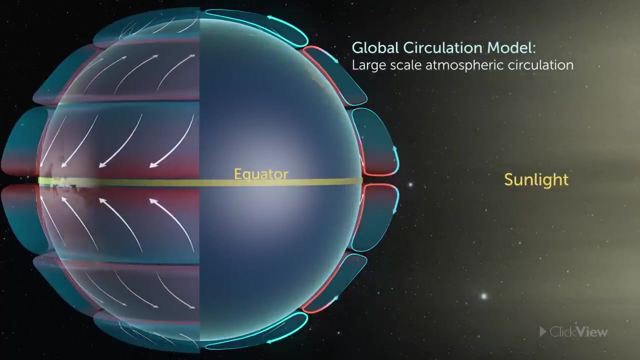 While storms are raging in the North Atlantic, in February in the Southern Hemisphere, Central Australia can be suffering intense heat and heavy tropical rains might be falling in the Amazon rainforests. The Global Circulation Model explains the Earth's atmospheric circulation, Heating and cooling. 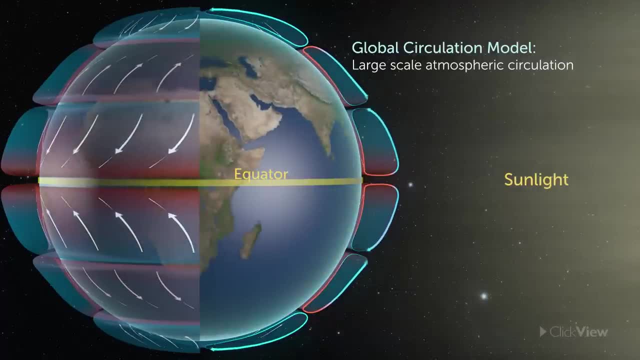 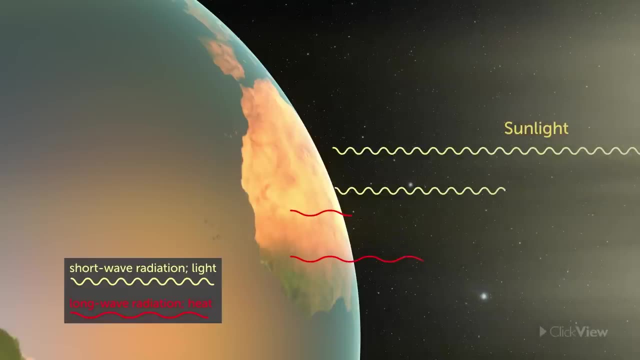 effects around the globe are driven by wind. The starting point of this model is heat from the sun. Energy from the sun is shortwave light radiation and not actually heat. The heat we feel comes from light absorbed on the Earth's surface, which is converted into longwave radiation that we feel as heat. 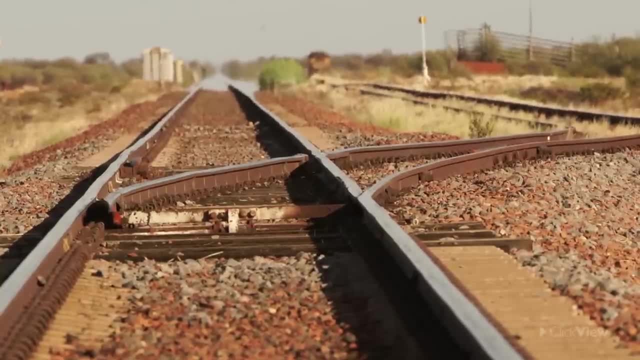 So, on a warm day, the heat we feel is due to the heat that we are body and mind. The heat we feel comes from light absorbed on the Earth's surface, which is converted into longwave radiation that we feel is heat. the heat we feel comes from the Earth's surface, heating the air around it. 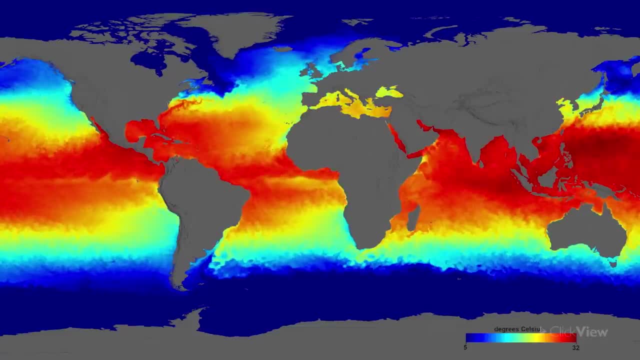 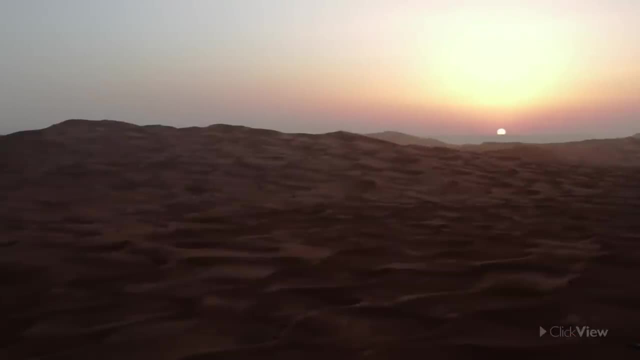 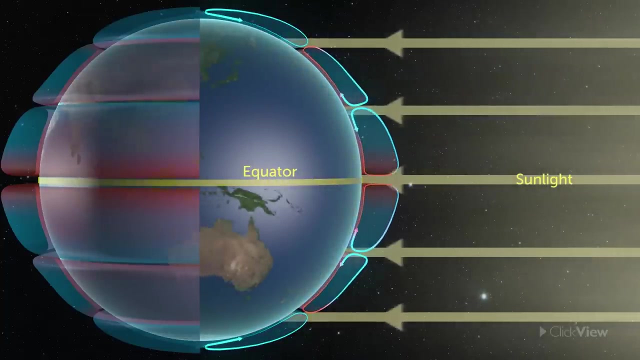 Our location on Earth plays a major part in determining the amount of heat we feel. In the Sahara, during the hottest months, air temperatures can rise above 50 degrees Celsius Over the course of one year. the intensity of solar radiation or insulation 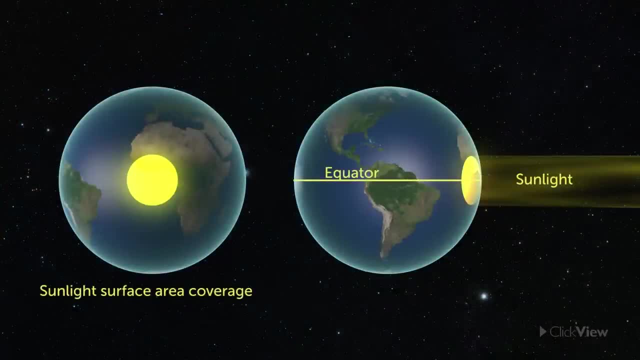 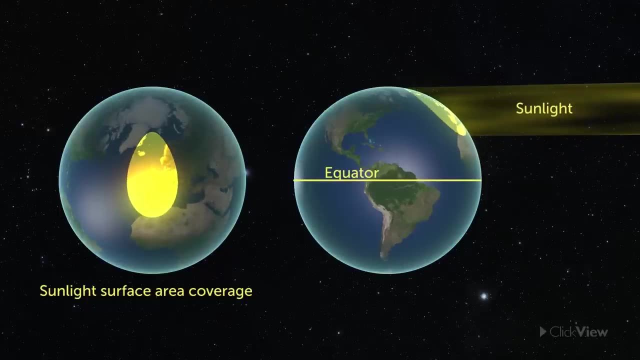 is greatest over the equator because the Sun is directly overhead At the polar caps. the Sun hits the Earth's surface at a much lower angle, so the same amount of energy is spread over a much larger area, which means it's cooler.